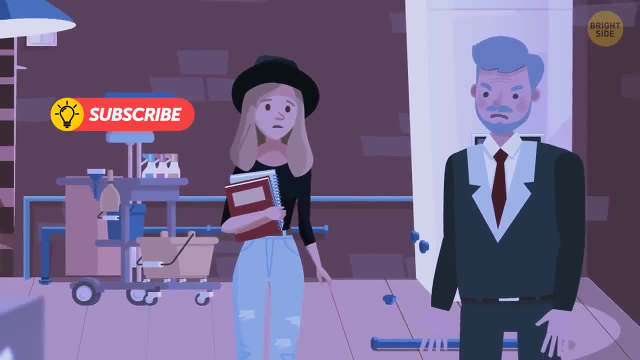 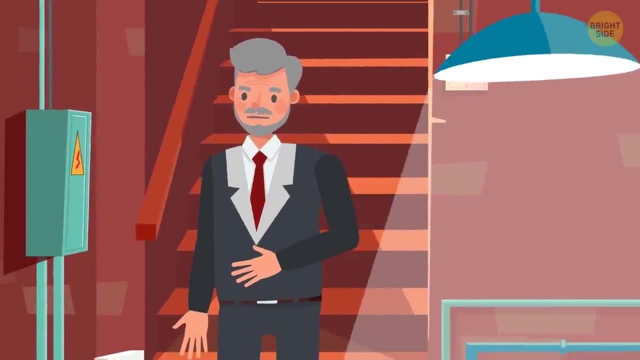 But why did she leave? Why did she leave? Why did she do it? Maybe she wanted to disrupt the physics? final, He turns the power back on. Ugh, hungry- Probably a good time to grab a quick snack. When he gets to the cafeteria, there's a new problem waiting for him. 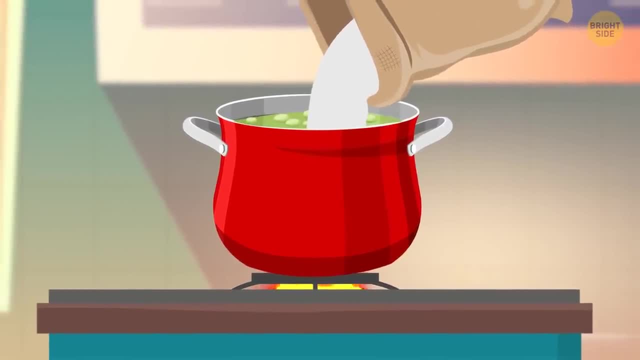 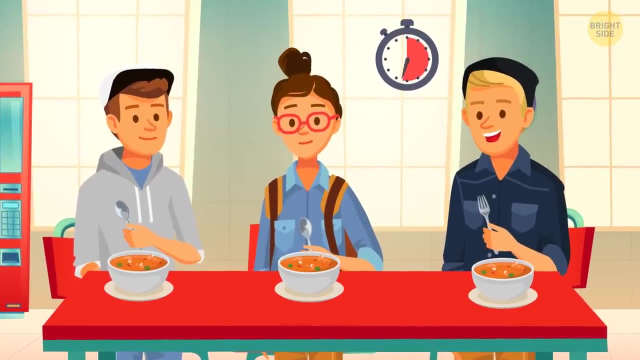 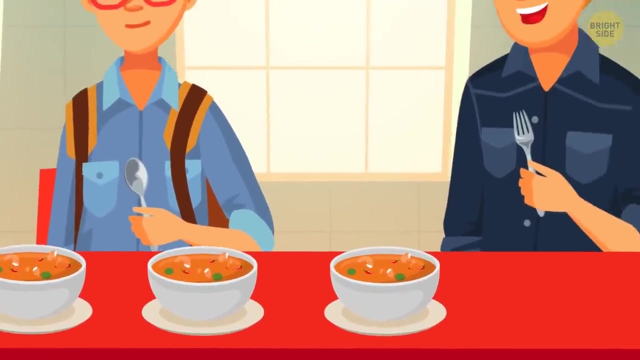 Someone emptied a whole bag of sugar into a huge pot of soup. Which student was it? You have seven seconds. All the suspects have left. They have bowls of soup in front of them, But one of them doesn't have a spoon, Just a fork. 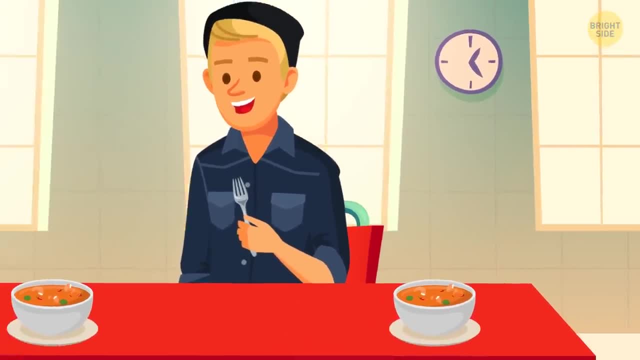 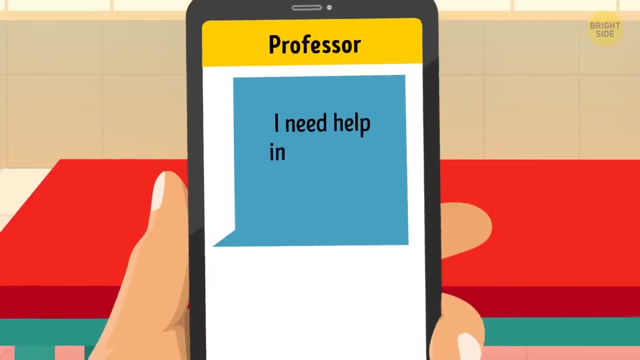 He was never going to eat the soup. He knew it would taste disgusting. Just as the president finishes up his sandwich, he gets a text. It's from a professor. He needs help in his office ASAP. In the office are three students standing around and looking guilty. 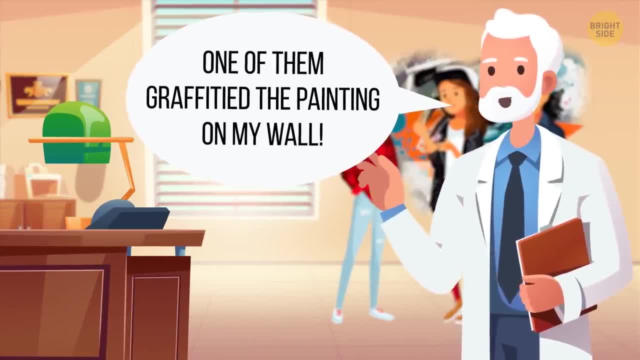 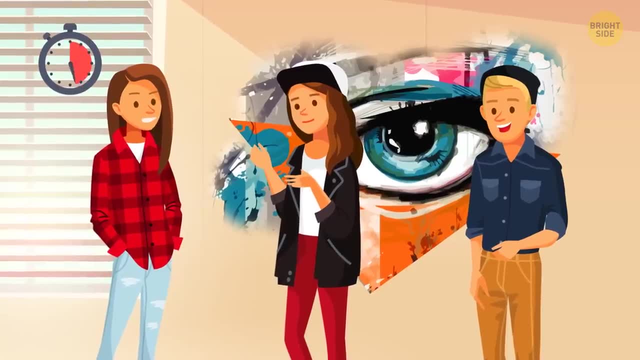 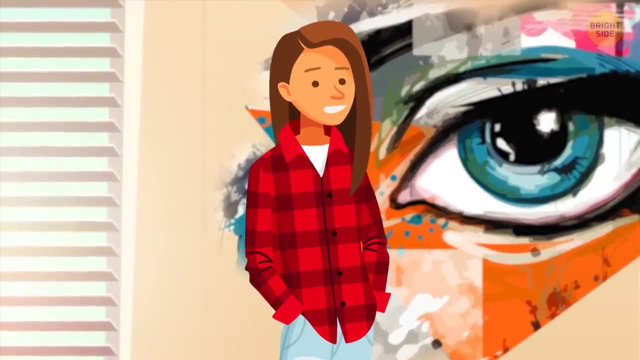 The professor claims one of them graffitied the painting on his wall. Which one did it? You've got seven seconds to figure it out. It's that one. She's covering her hands. There's probably some paint on her fingers that she's trying to hide from you. 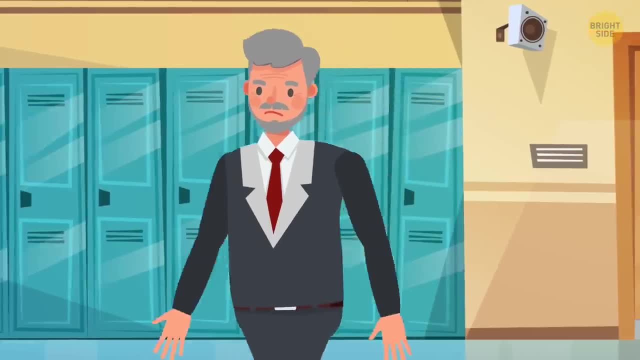 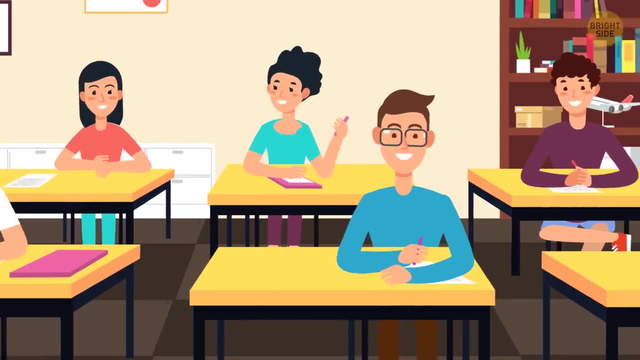 Next stop, the infamous physics exam. The president heads over to the exam room. Everything's quiet in there, Looks okay. All the students have their heads down staring at their papers. But someone's cheating. The president can sense it somehow. 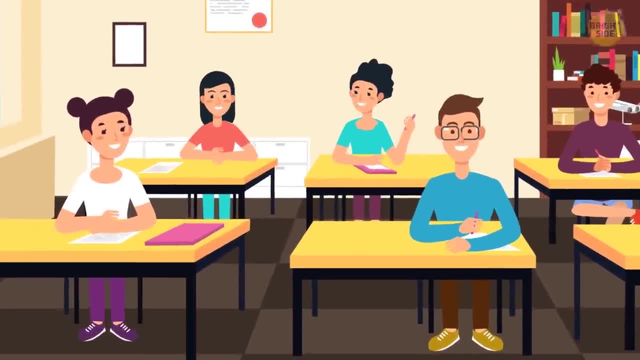 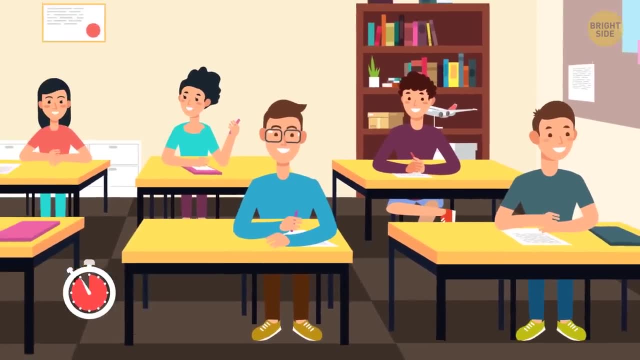 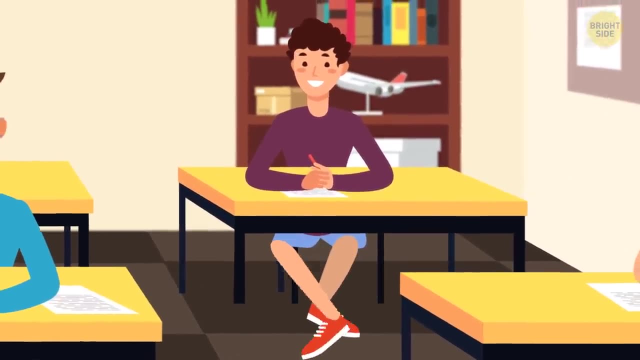 Help him find the sneaky student. Seven seconds to scan the room. It's the guy with his legs crossed. Clever, He wrote the answers on his calf muscle, But where did he even get those answers? After a brief shakedown, he spills the beans. 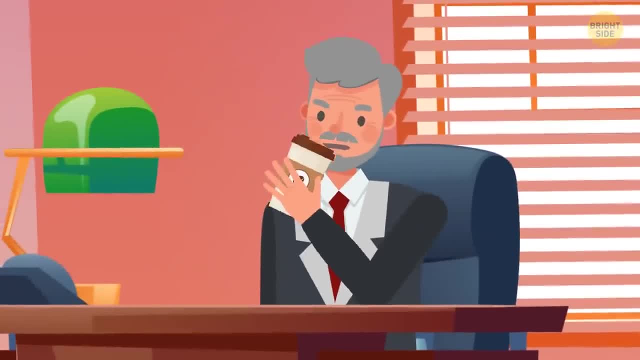 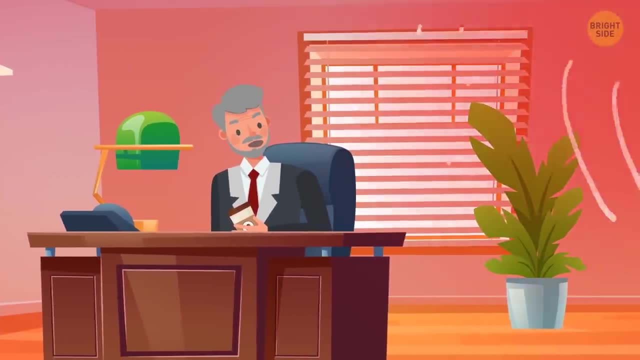 He got them from a friend That hassle's over Time for a coffee and a snack- A big one. But just then a piercing beep smashes through The silence. The fire alarm. Oh, come on. Students file out of their classrooms and the entire university has to be evacuated. 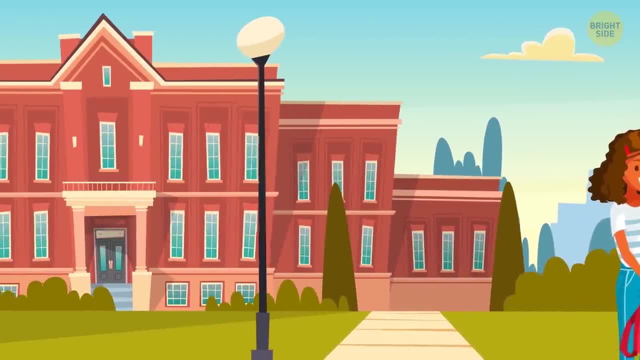 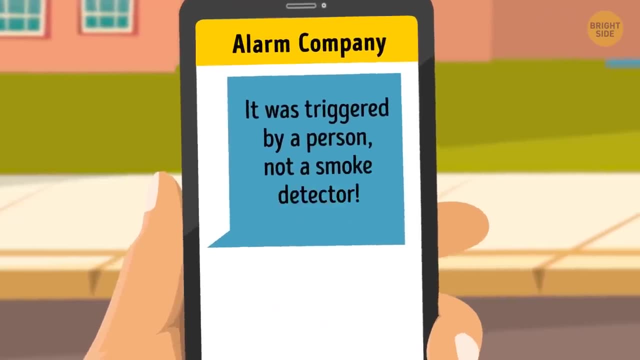 The students are standing outside looking at the building. No fire, No smoke. even The president gets a text from the alarm company. The alarm was triggered by a person, not a smoke detector. The president looks around Time to round up the usual four suspects. 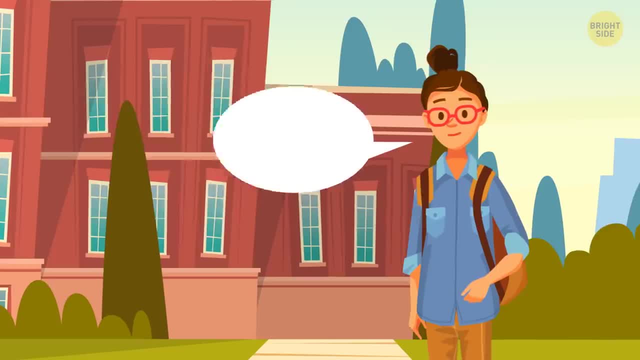 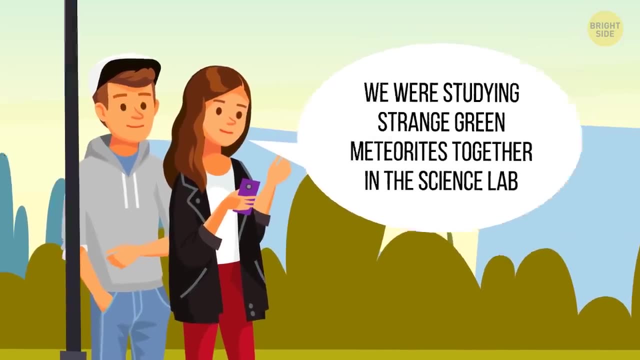 Matt says he was in the bathroom when the alarm came on. Julia Was taking the geography final. Clark and Lex were studying strange green meteorites together in the science lab. Which one of them is lying? You have seven seconds, starting now. 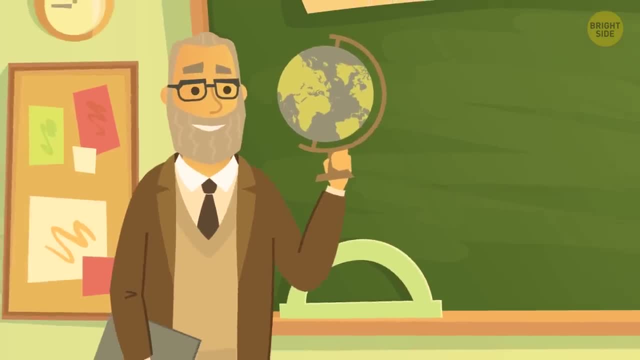 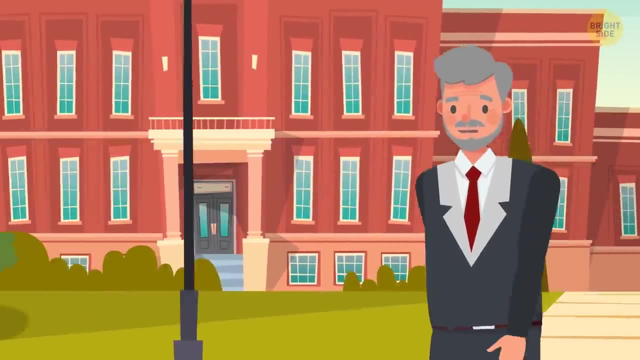 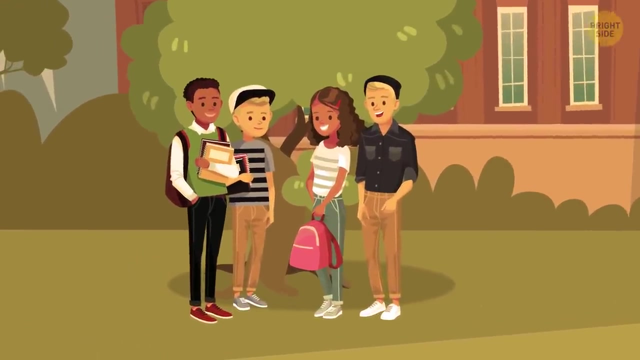 It was Julia. The geography teacher postponed the final remember. Why would she lie unless she had something to hide? Today's- not really his day. Someone cut down a tree Right in the middle of the quad. The caretaker saw four students hanging out under the tree this morning. 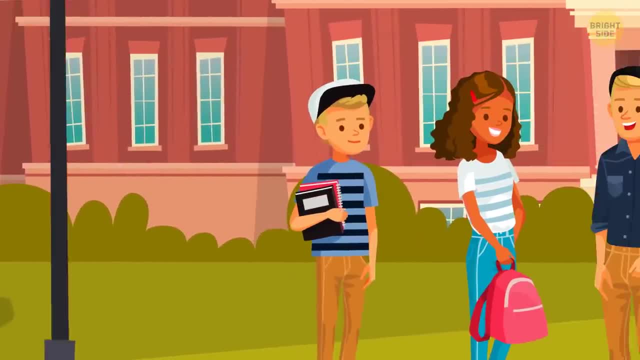 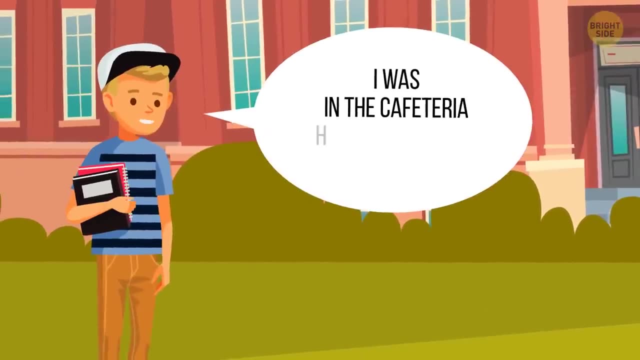 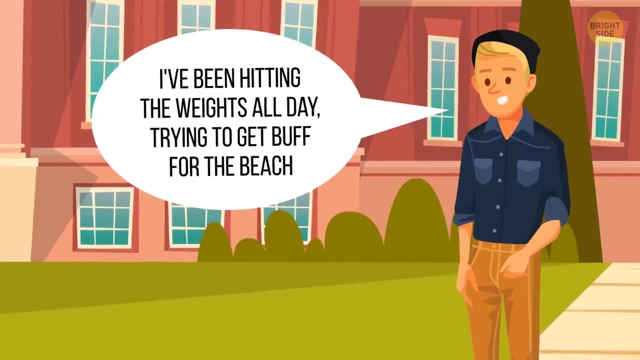 And now it's gone Time to interview the suspects. Emily says she's been in the library all day. Loads of people saw her. Sam claims he was in the cafeteria having some soup, Louis was in the physics final And Michael says he's been hitting the weights all day trying to get buff for the beach. 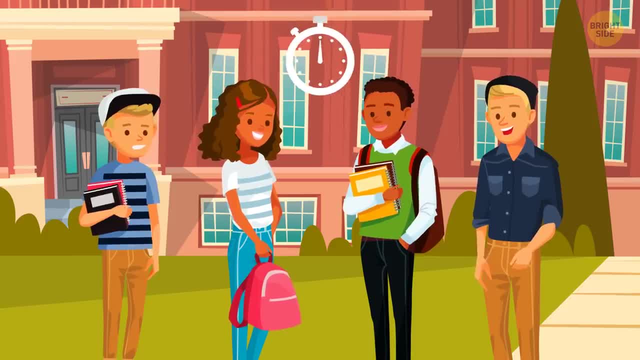 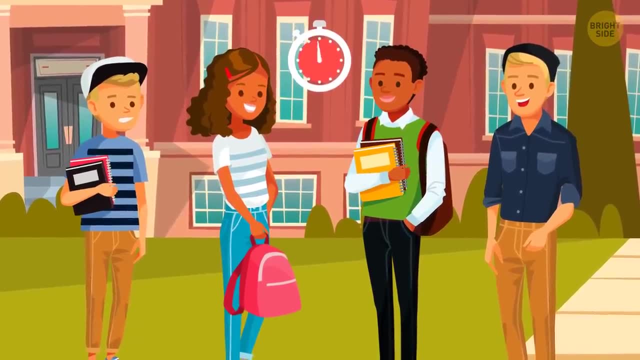 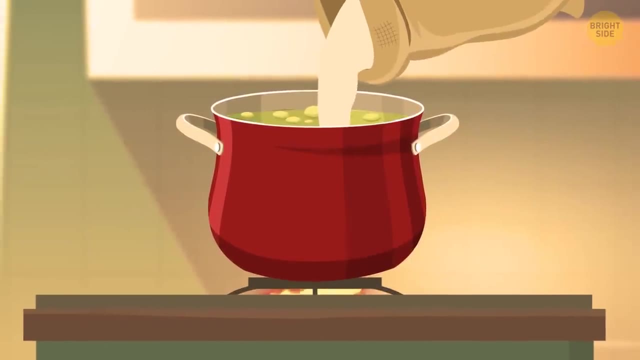 Who cut down the tree? Your seven seconds starts now. It was obviously Sam. He said he was having some soup, But remember, If he had really been in the cafeteria he would have mentioned the whole sugar thing. Plus, the president was in there and didn't see him. 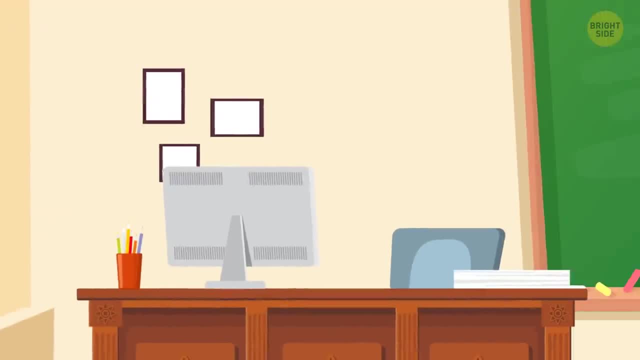 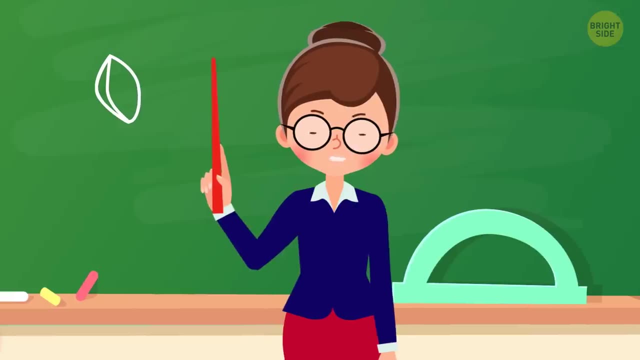 He's lying On to the biology final. They've got a new teacher who's giving a unique type of final. The president sneaks in the back of the room. The teacher explains that She gave her students ficus seeds at the beginning of the semester. 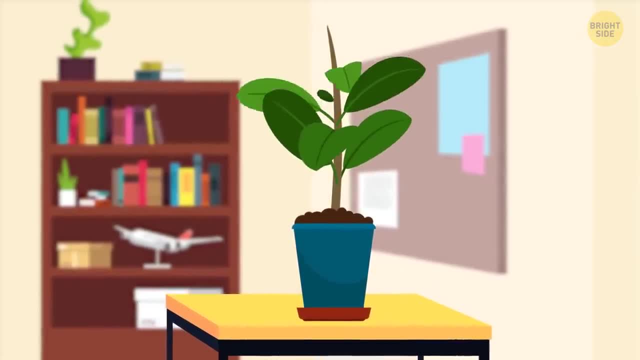 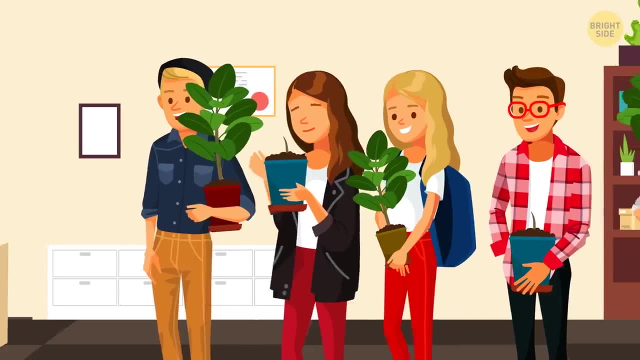 Whoever has the most beautiful ficus plant will get the highest grade. It's time to present the results. The students start to file into the classroom. Half of them are holding pots with beautiful green ficus trees. The other half have pots filled with plain old earth. 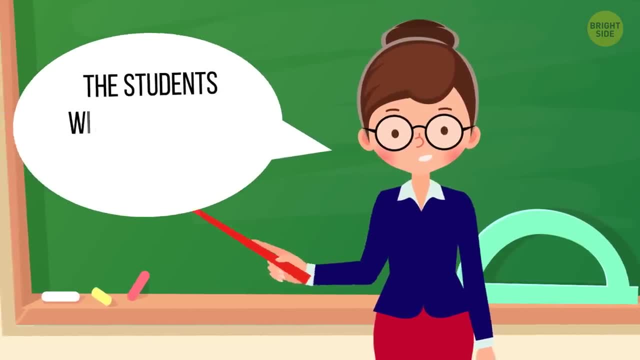 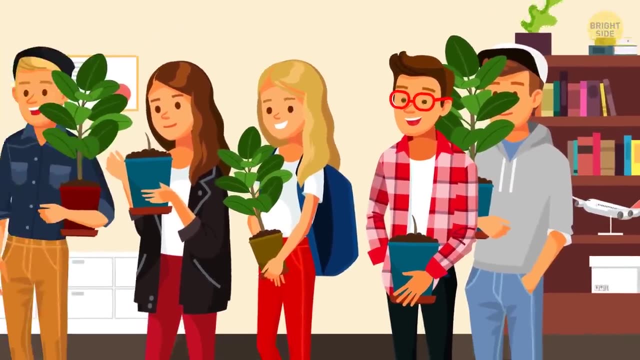 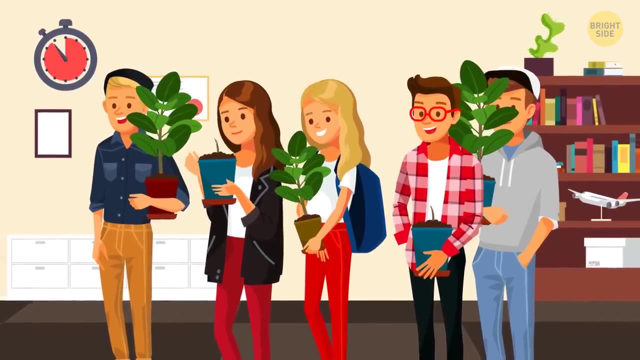 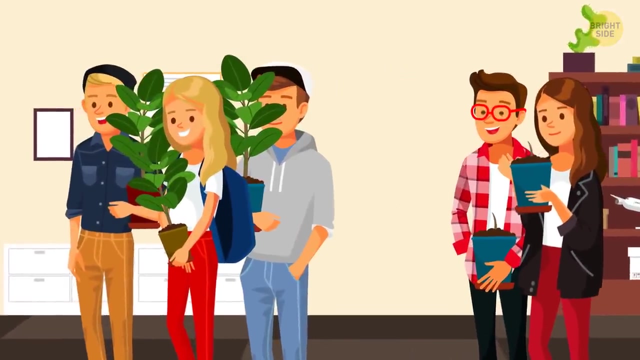 No leaves no nothing. The teacher says the students with empty pots all get an A. Why did the teacher do that? Solve this mystery in seven seconds Go. At the beginning of the semester she gave everyone fake ficus seeds. The students who showed up with full blooming plants must have bought a full-grown plant and stuck it in the pot. 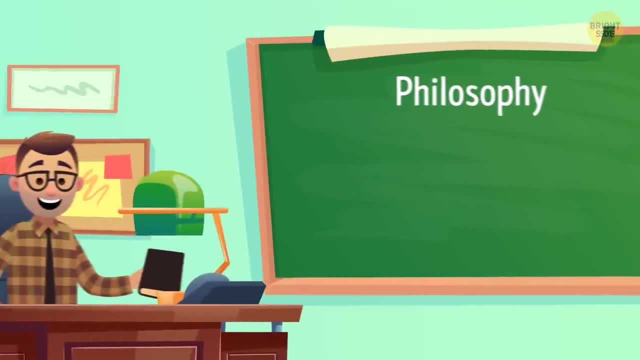 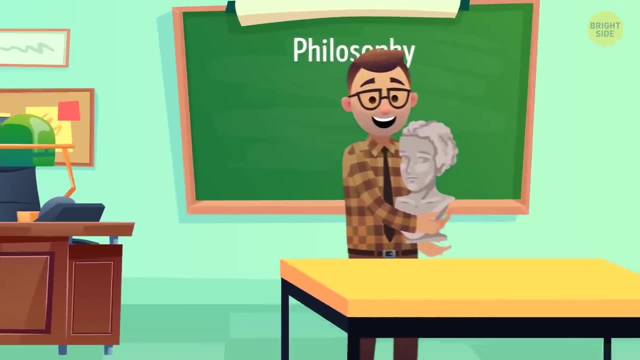 Ha Busted. Last final of the day: philosophy. The young teacher is in there waiting for all the students to take their seats. After that he puts a bust of an ancient Greek philosopher on the table. The teacher says: Write a short essay on the following topic. 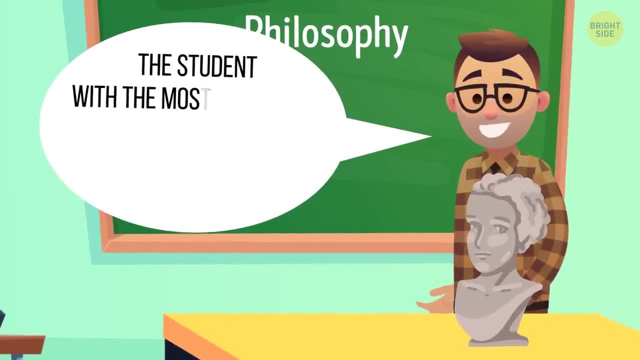 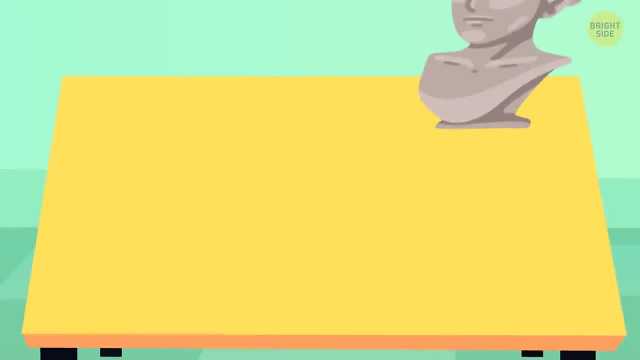 Why this bust doesn't exist. The student with the most convincing argument gets an A, while everyone else gets a C. Ha, Tough teacher. After an hour, the students hand in their papers, Most of them filled up the front and back. 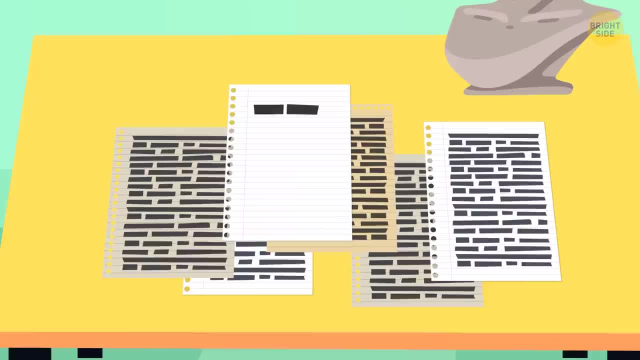 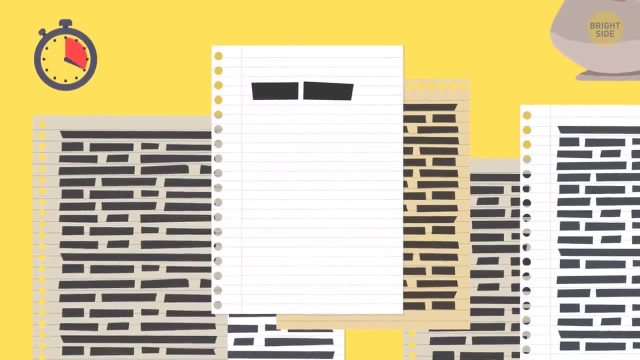 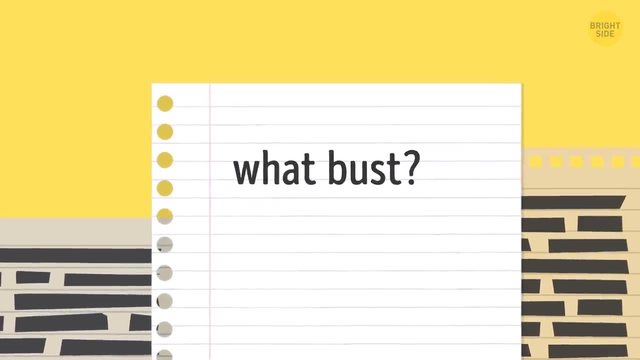 but one student only wrote two words and she got the A. What did she write? I'll give you seven seconds to figure it out. She wrote: What bust The president heads outside again, this time for the parking lot. What? 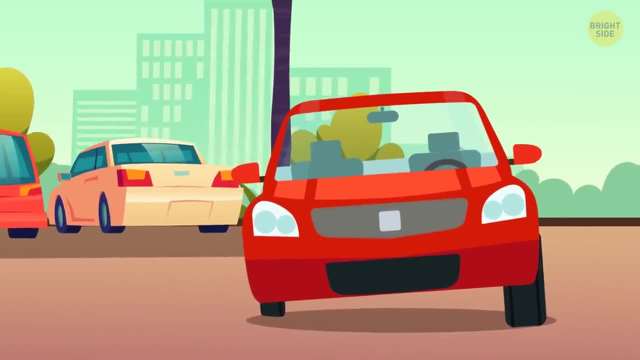 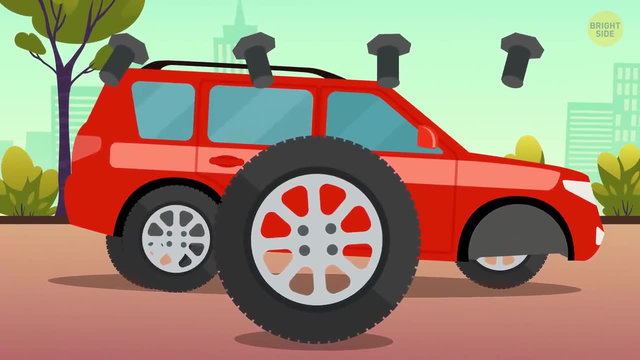 Someone took the tire right off of his car. How's he gonna get home? He still has a spare tire in his trunk, but the thieves took the bolts too- All four of them. What can he do? You have seven seconds to come up with a plan. 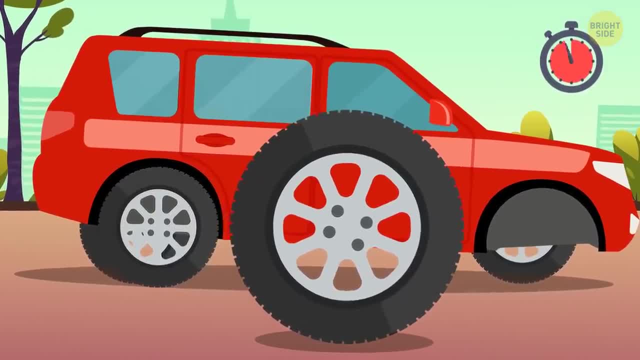 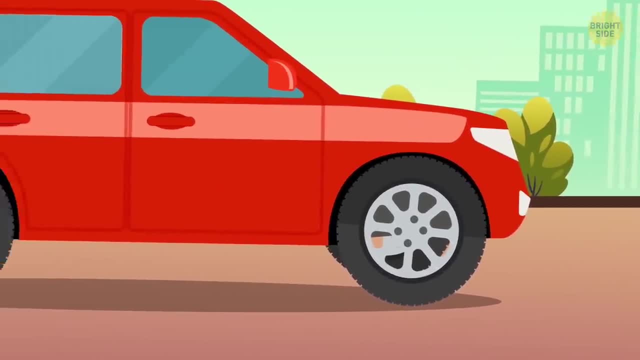 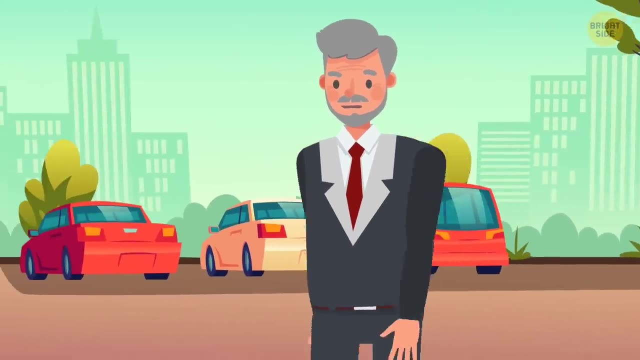 He needs to unscrew one bolt from each of the other three tires and attach them to the spare. Each tire now has three bolts. That'll be enough to get to the nearest service station. What an intense day. The president's ready to kick back for a few? 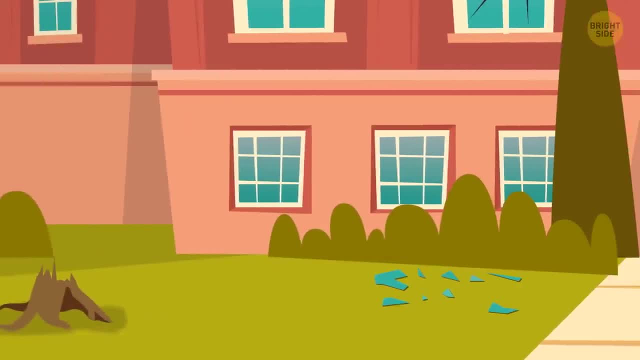 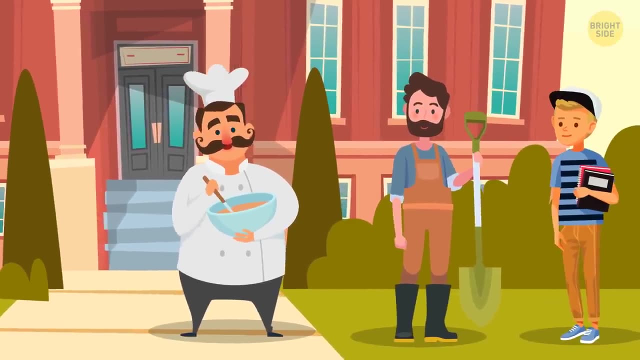 but he gets another urgent text. There's broken glass all over the quad. Someone broke a window up there. The only three people around are a cook, a gardener and a student. The cook says he's been boiling up a new soup for the last hour. 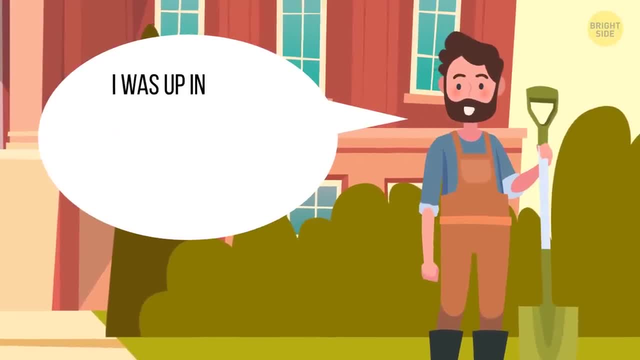 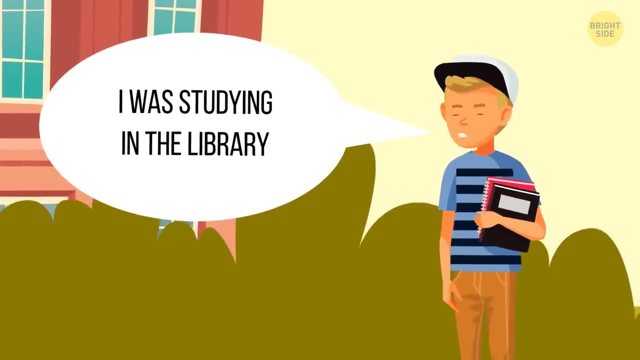 since someone put sugar in the last one. The gardener admits he was up in a tree cutting branches. He saw a student break the glass. The student says he was studying in the library. I'll give you seven seconds to figure out who's lying. 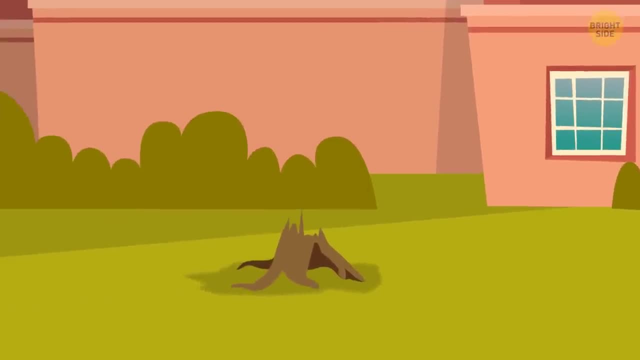 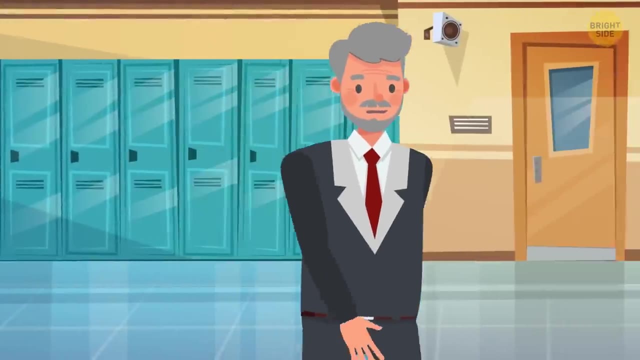 The gardener's lying. How could he have been up in the tree? He'd had already been stolen. He broke the glass, probably just by accident. The day's finally over. The president heads over for the best tradition on campus: the post-finals party. 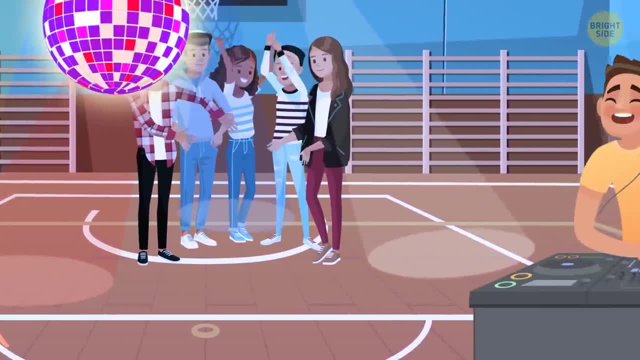 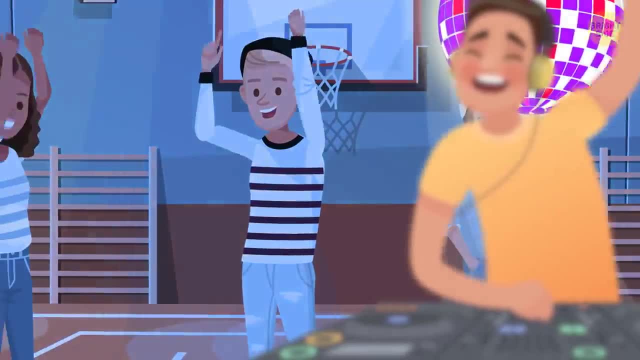 It's in the basketball arena. There are lights, decorations and even a DJ. Everyone's dressed up, looking relieved. Finals are over. The party goes all night, but around 4 am someone accidentally slams the doors too hard. 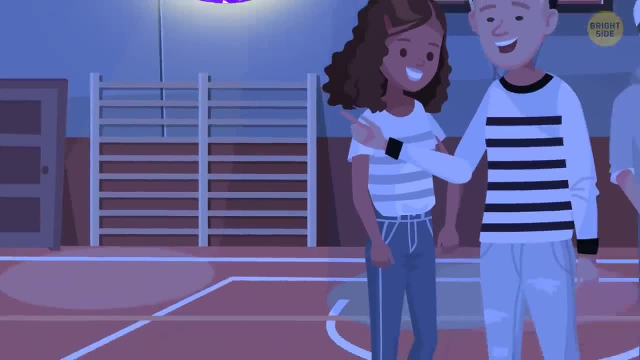 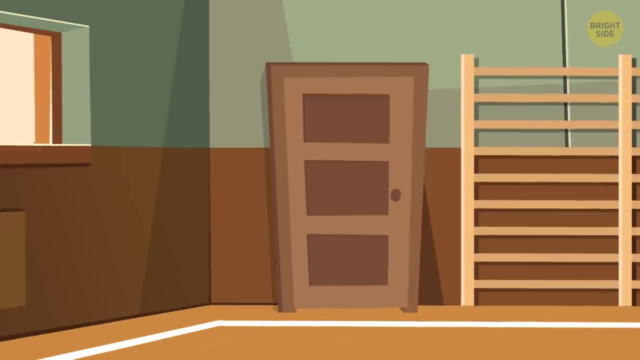 and it triggers the automatic locks. Everyone's trapped. The president can be the hero of the party. He just needs to find a way out, grab the spare keys from his office and open the door from the outside- But how? One of the students, Eric. 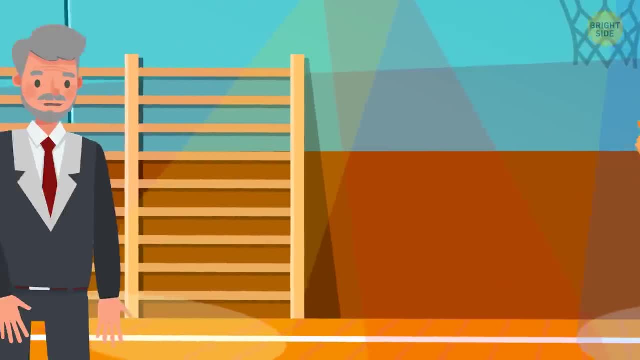 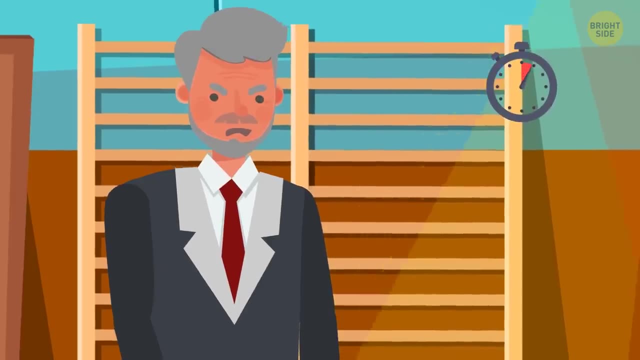 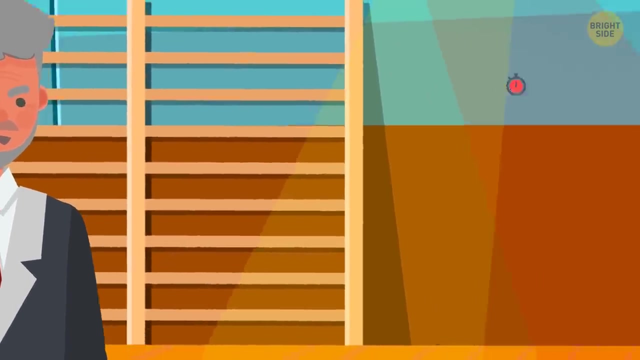 says he knows how to get out of the gym through a vent. The president looks at him and his face goes red with anger. Why Last riddle Seven seconds? You can do it. Eric just gave himself a chance. He's obviously been in the ventilation shafts before. 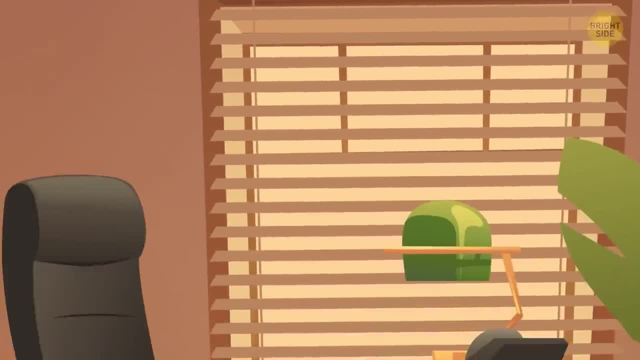 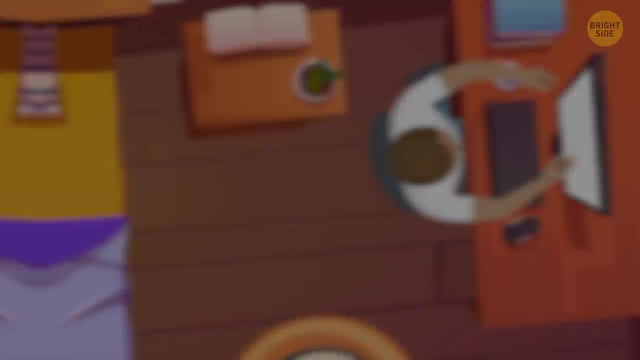 so it was probably him who stole the physics final. How did you do Count up your correct answers and let's see how you fared on your final exam: Zero to three points. Eh, looks like you'll need to sign up for some classes over break. 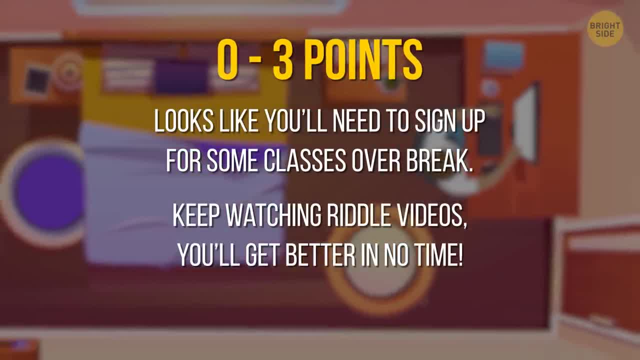 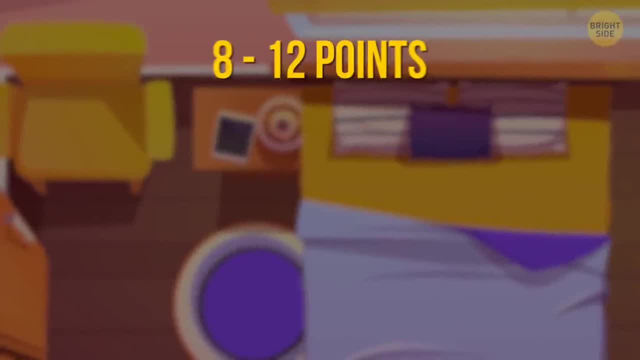 Keep watching riddle videos, You'll get better in no time. Four to seven points: Solid B plus, But I'm sure you can do better next time. Eight to 12 points: You nailed that. four to 12 point Final. Leave your books in your locker and enjoy your well-deserved vacation.